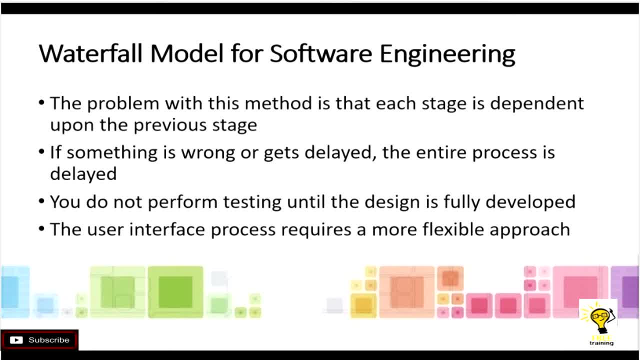 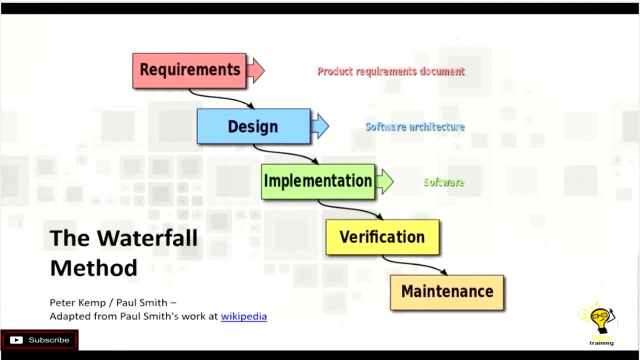 final step is testing and you find out it's completely incorrect. This is what the waterfall method looks like, And this is adapted from Paul Smith's work at Wikipedia, At least this particular diagram of the waterfall method is. So you can see we have requirements, then the design, then the implementation, then 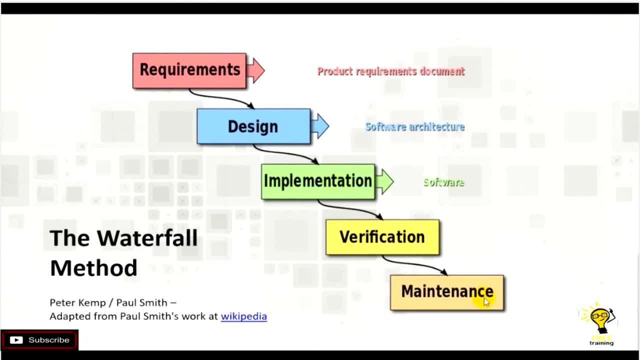 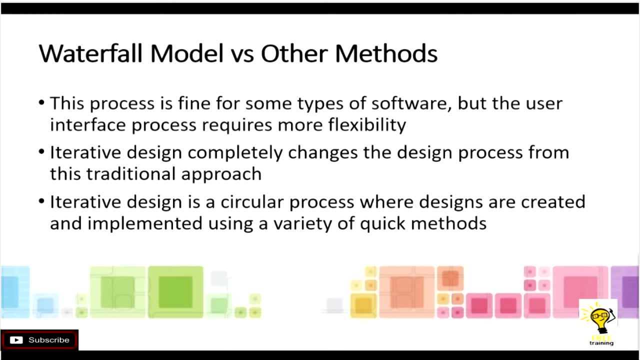 verification and then maintenance, And every method is dependent upon the prior phase. This process is fine for some types of software, but the user interface process requires much more flexibility. Because of that, iterative design is what's preferred, And this completely changes the design process from the traditional waterfall model. 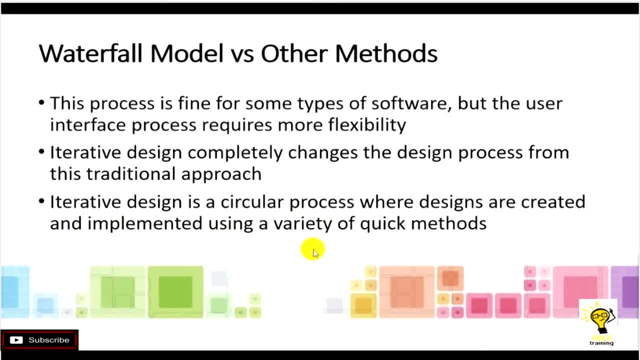 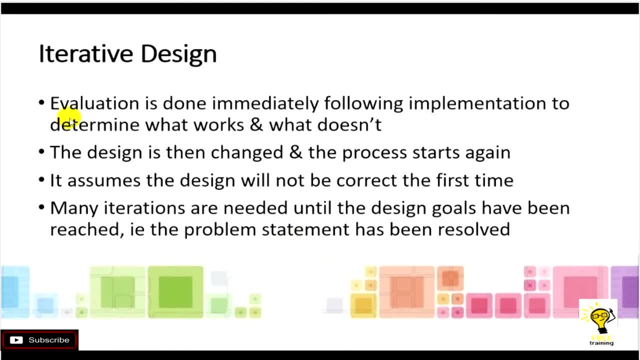 Iterative design is a circular. Designs are created and implemented using a variety of quick methods. The benefit of this is evaluation is done immediately following implementation to determine what works and what doesn't. You're checking on that throughout every portion of iterative design. 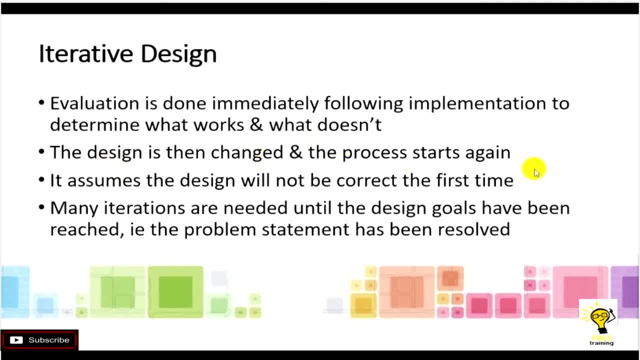 When you find out what doesn't, the design is changed and the process starts over. So this is very circular. It assumes the design will not be correct the first time, which is rather unusual. It was a novel concept when it first came out, as you can see, compared to the waterfall. 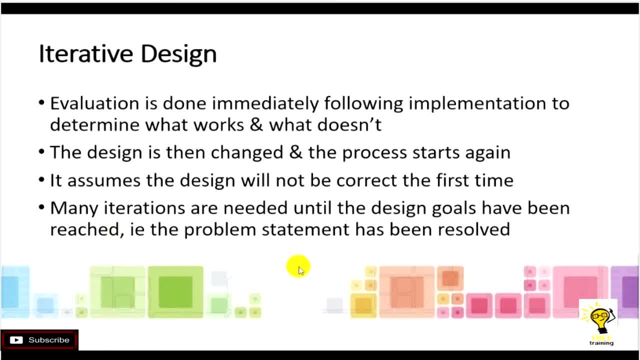 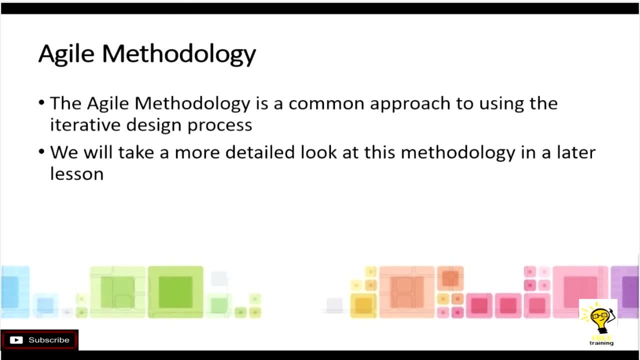 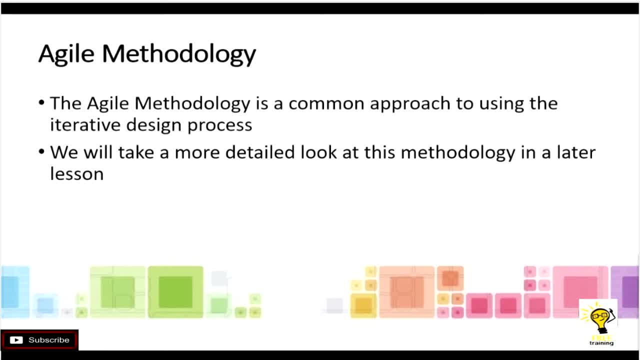 It's a common approach to using the iterative design process, So this is one methodology that is commonly used within that process. We're going to take a look at that agile methodology in a separate lesson, But the agile methodology within iterative design is one of the more common approaches. 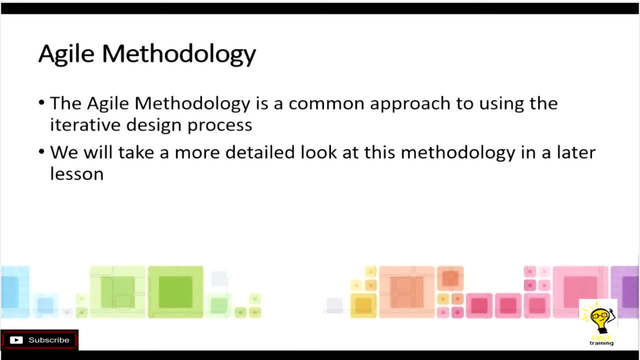 to working with UI design, So that's information about the value of iterative design And how it's used and considered to be best practice for user interfaces. We'll be looking at the agile methodology within this approach And we'll address the details of agile methodology in another lesson within this course. 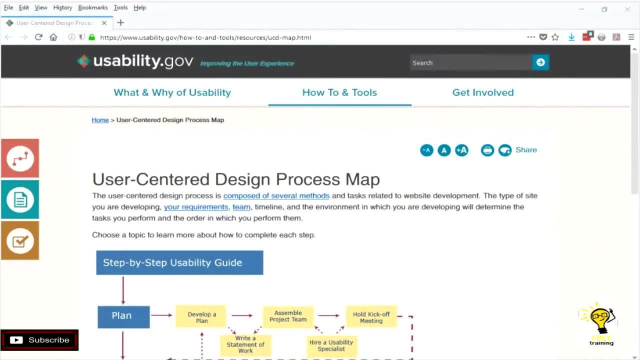 In this lesson we're going to talk about the user centered design process. Now there is a special type of iterative design. It's called the user centered design process. This process is a widely accepted way to build user interfaces with good usability properties. 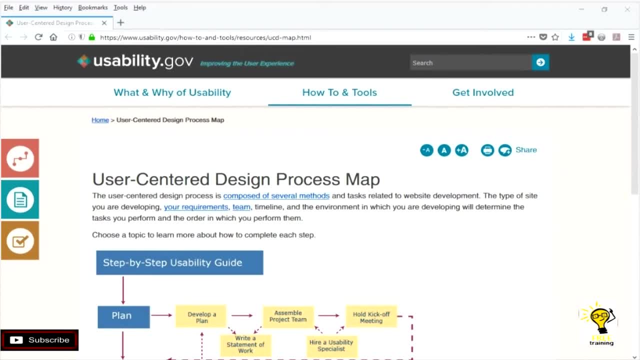 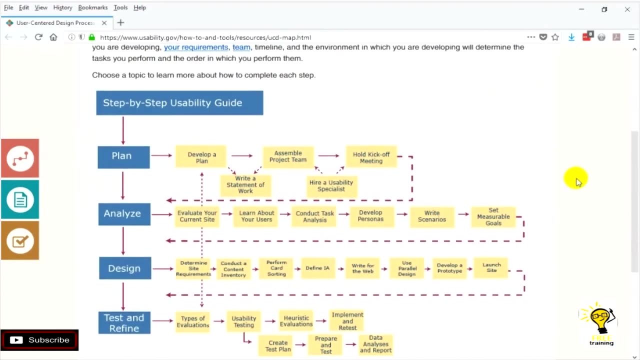 Because when we're designing an interface, we have to make sure it's usable to a user, of course, And usabilitygov has an amazing process map that explains the process. And it doesn't just explain the process, What it does, It actually allows you to click on any pieces within the process and get more information. 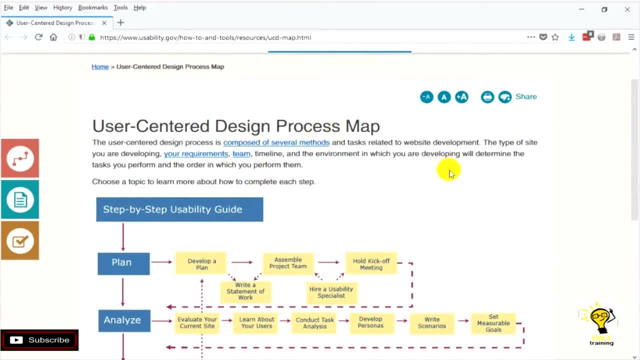 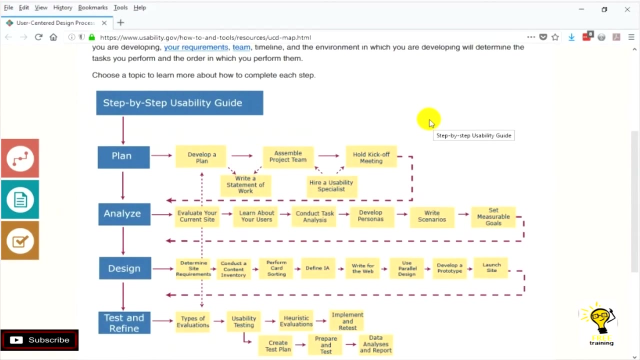 about it. So this is a design process map for user centered design. There are several methods and tasks available, But this particular one keeps the user at the center and focus. So the idea is you first have to come up with a plan. 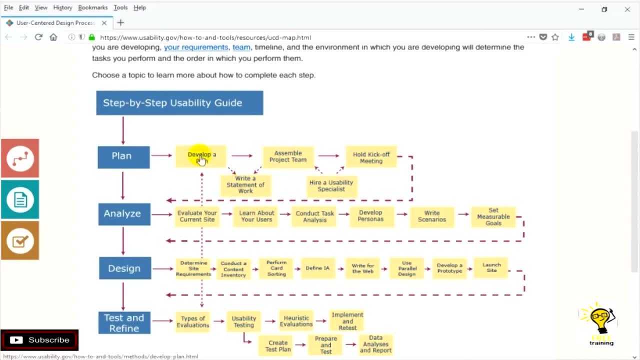 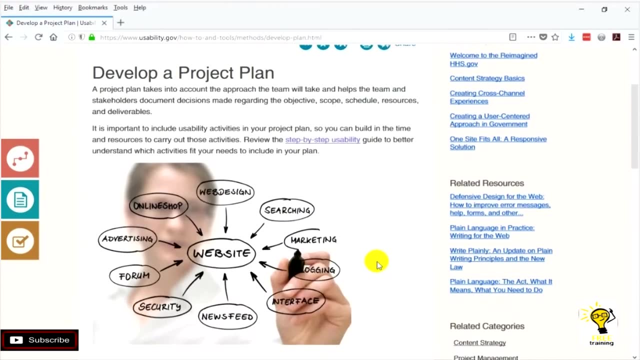 So these are the steps for developing a user centered design process. So if I want to understand that, I'll click on develop a plan, And here is information that starts to walk me through the steps, And there's even a step by step usability guide for creating a project plan. 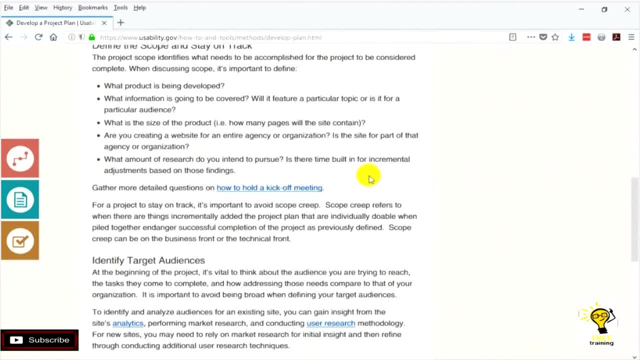 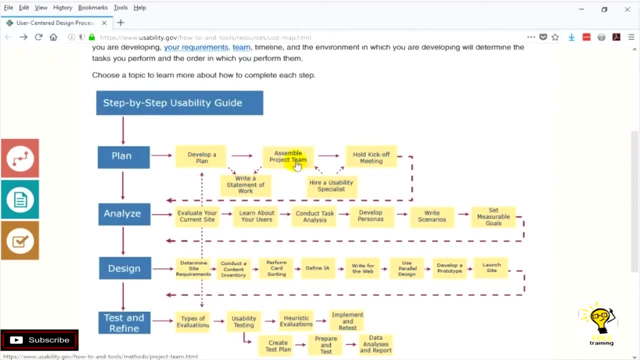 The things you need to do within it. This site really is amazing because it walks you through the information for each step. You can assemble a project team, hold a kickoff meeting and you have some other steps inside of that. Now notice these blue options. do not have clickable links on them. 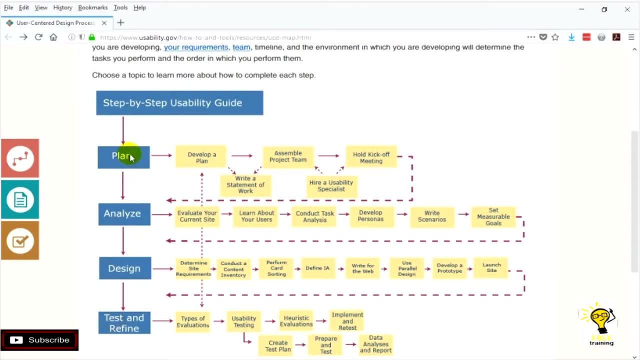 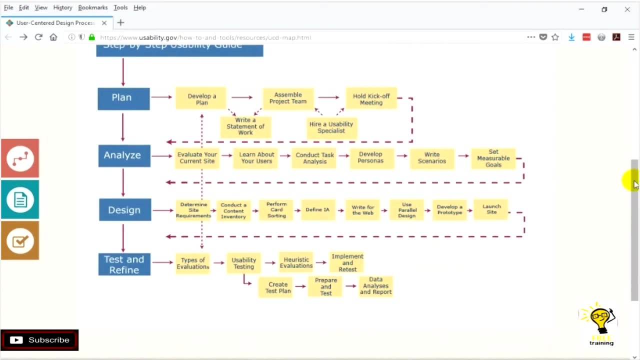 So these are the steps required And then, within each step, these are the individual tasks. So everything in yellow is a task that you can click on to find out more about it, And analysis That is coming up with data analysis to figure out what it is you want to be doing and what your users are. 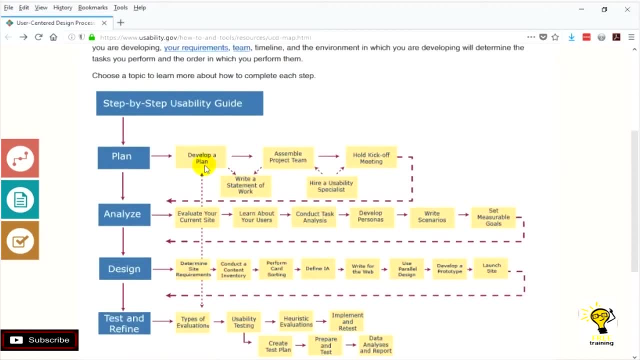 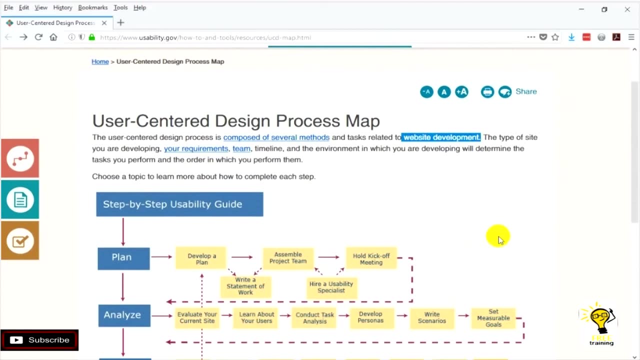 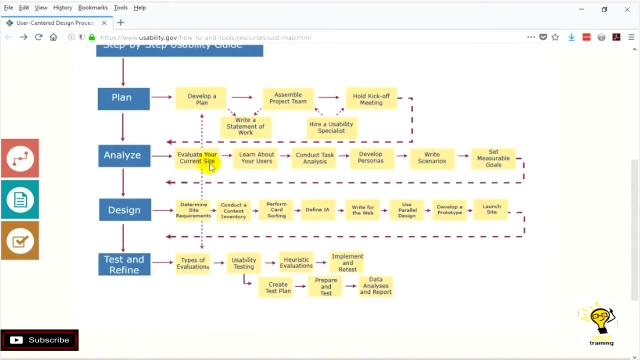 presently doing. notice: evaluate your current site. now up at the top it does say website development, but this concept is exactly the same, even if it's not a website. evaluate your current app. if it's an app you're building, learn about your users. what are the different ways you can go about doing that? I'll click. 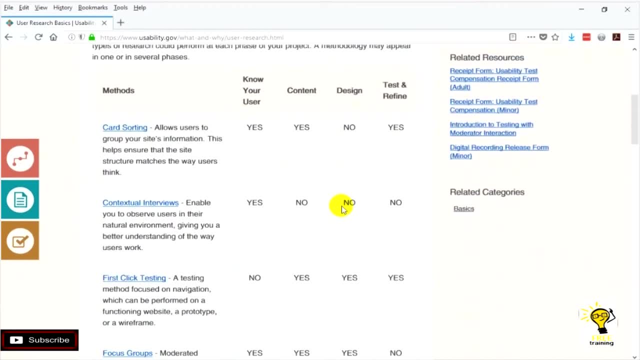 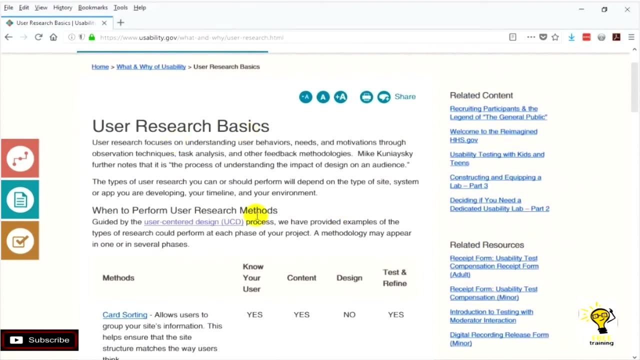 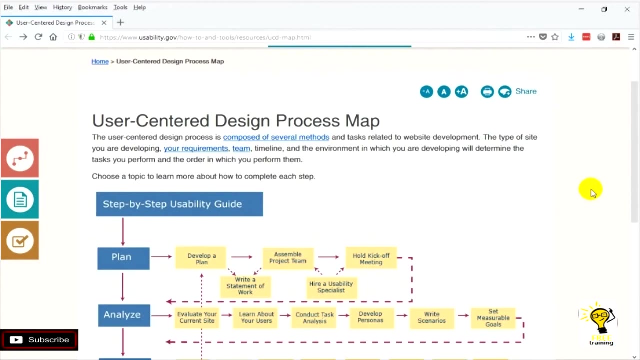 on that one: user research basics. we looked at this particular link earlier in the course. this is describing all of the different user research methods that are available and what specifically they're good for in the process. this process map to me is really amazing. you can even print this map, so you have it. 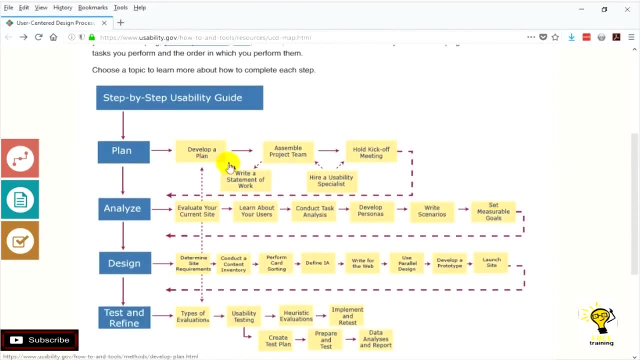 available. but what's nice about it as a URL? you can even print this map, so you have it available. but what's nice about it as a URL is each one of these are clickable, so as you move through each phase of this user-centered design process within the iterative design methodology, you have 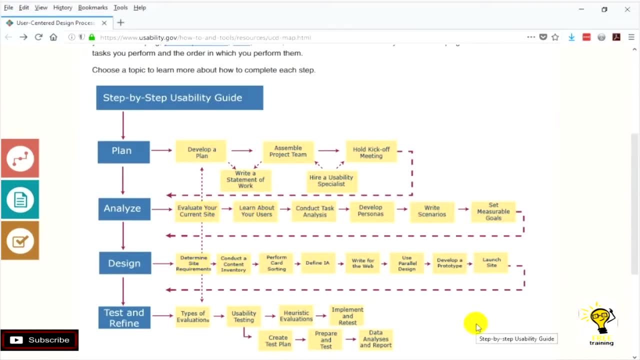 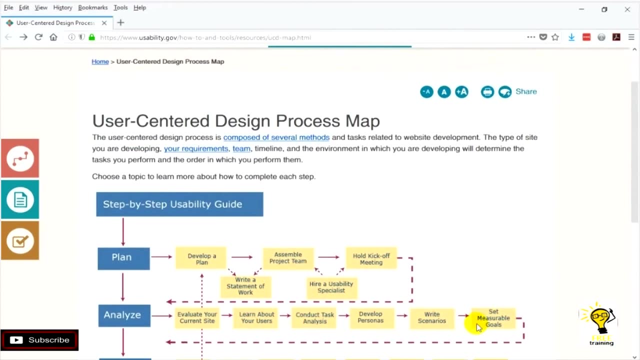 access to a lot more information and you can make sure you're following the steps accordingly. so this process map is a very valuable tool for making sure you remain within the user-centered design focus and are using an iterative design process, so that is user-centered design. the 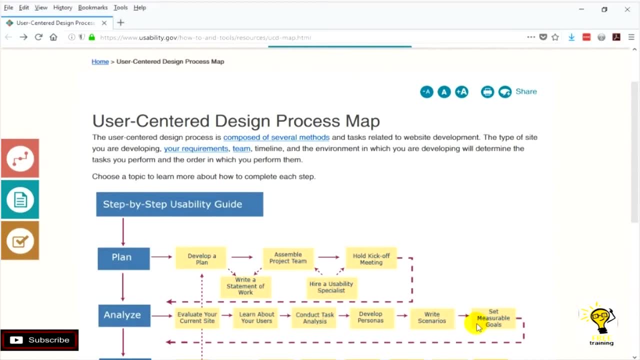 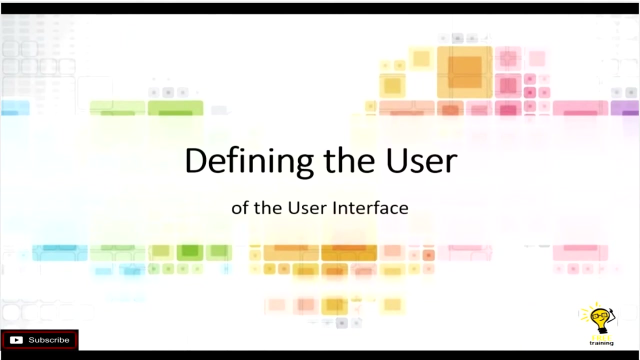 process available within that, and also all of the various steps, along with details about each step along the way, to make sure that you are following and incorporating everything that needs to be done to make sure you are using a user-centered approach to your UI development. when working in UX and UI design, we are supposed to keep the user at the center. 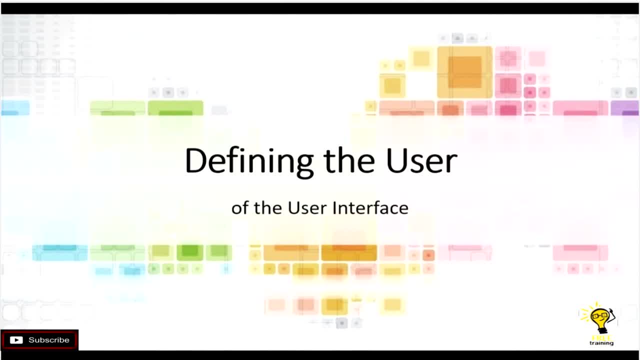 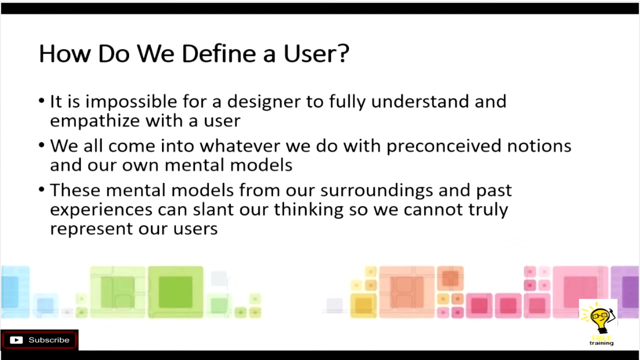 of the design process, and that's great for the process. but how do we define that user? we want to keep at the center of the process, so this is going to look at defining the user of the user interface. so how do we define a user? a user is about to be the example of a designer that is ever going to be able to. 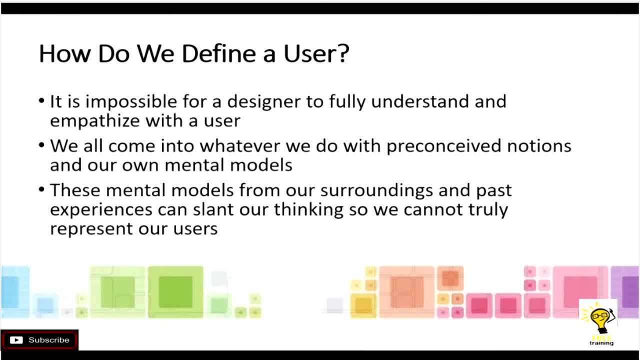 say: I'm not you. it is impossible for a designer to fully understand and empathize with a user, specifically because we are not them. we all come into, whatever we do, with preconceived notions and our own mental models. these mental models are from our surroundings and 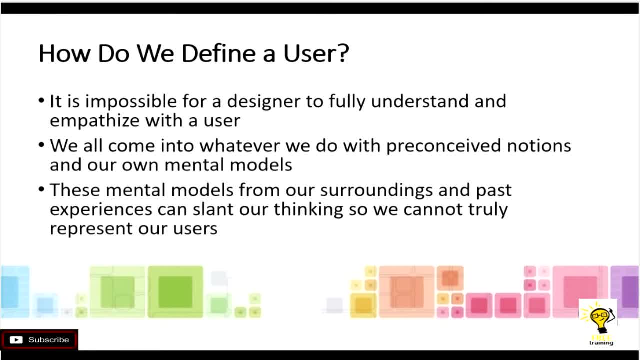 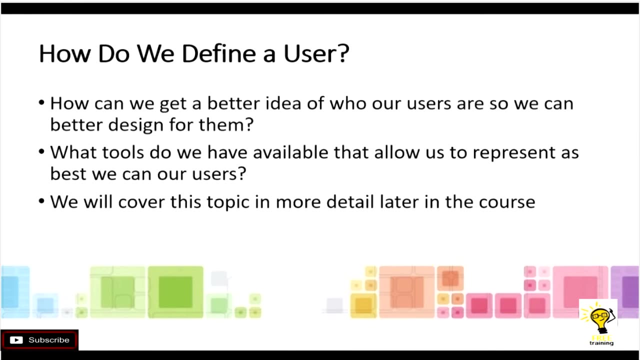 cannot truly represent our users as a designer. Users come into our user interface and our designs with their own preconceived mental models, And if our interface does not match their mental models that they came in with, they are not going to be comfortable in the interface. 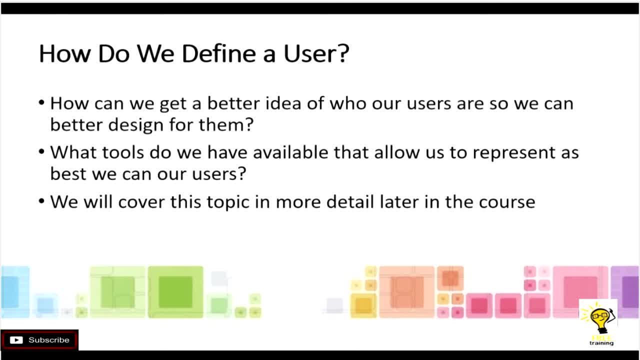 So how can we get a better idea of who our users are so we can better design for them? And, more importantly, what tools do we have available that allow us to represent as best we can our users, And that's as good as it gets. 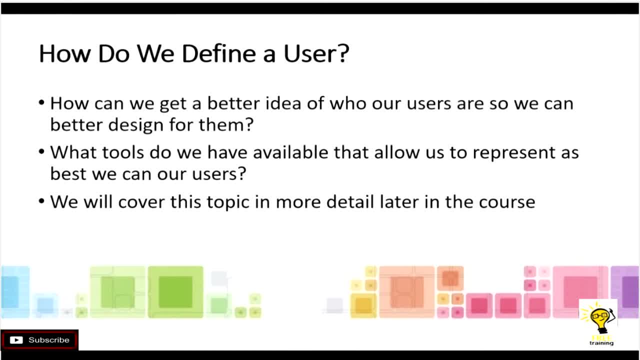 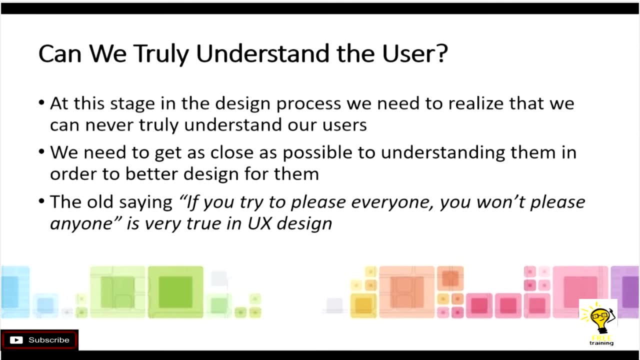 We're going to cover this topic in more detail later in the course with regards to the specific tools that can be used to assist you in that process. So, can we truly understand the user At this stage in the design process? we simply need to realize that we can never truly understand. 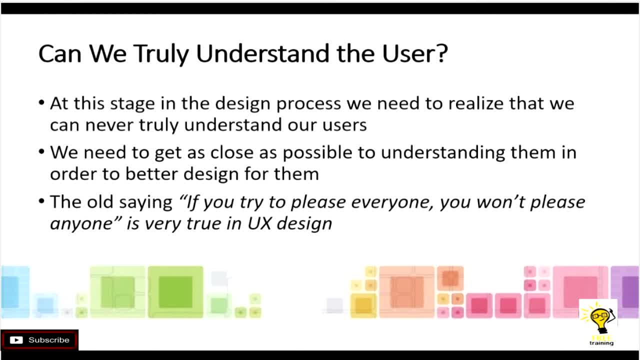 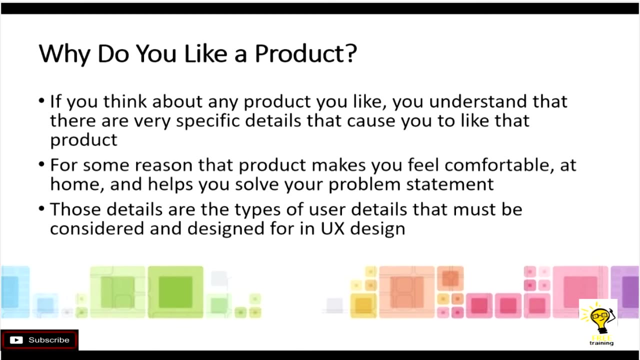 our users, but we need to get as close as possible to understanding them in order to better design for them. The old saying, if you try to please everyone, you won't please anyone is very true in UX design. So you do have to be very careful when defining that user and trying to understand them. 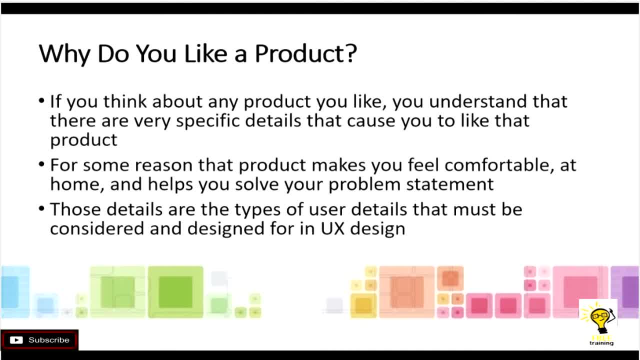 Why do you like a product? If you think about any product you like, you understand that there are very specific details that cause you to like that product For some reason. that product makes you feel comfortable at home and, most importantly, it helps you solve your problem. statement. 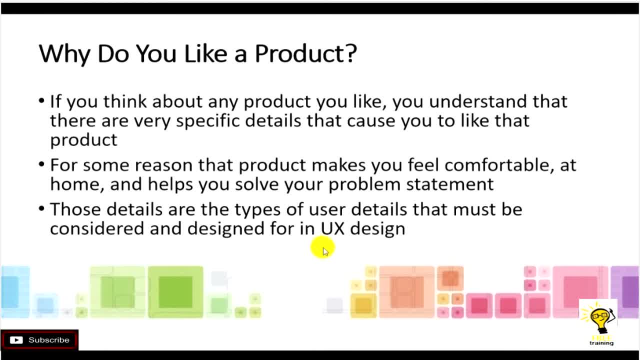 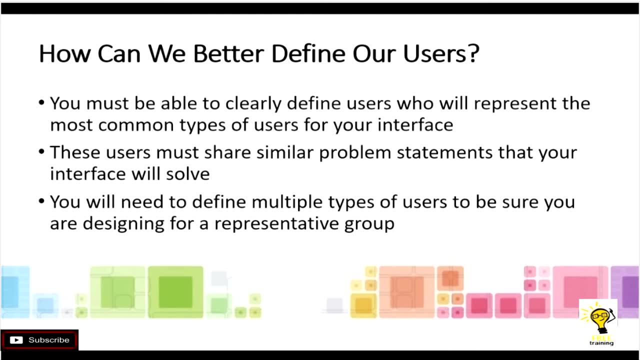 Those details are the types of user details that must be considered and designed for in UX design. So those are the details that you have to remember as a designer. So how can we better define our users? You must be able to clearly define users who will represent the most common types of users. 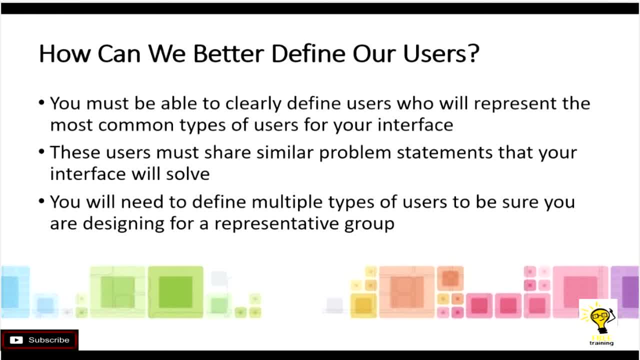 for your interface. These users must share similar problems. You must be able to clearly define users who will represent the most common types of users for your interface. You must keep in mind what kind of users you kids design for the unique issues you gotta address and get information fromoks to such consumers, who'll interpret them right and 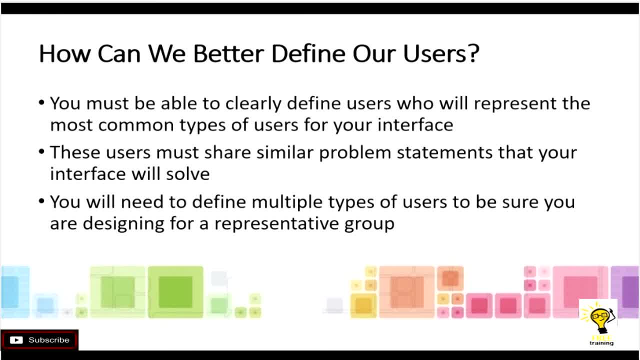 find the right response. So, even though the users may be very different, they'll already be coming into your interface with similar problem statements that your interface is going to solve for them. Because of that, you'll need to define multiple types of users, because you need to make sure. 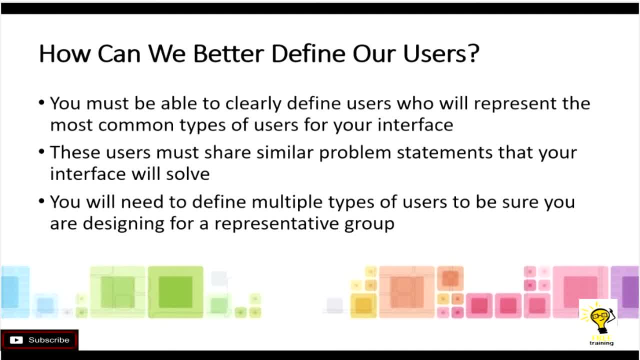 you're designing for a representative group. Just keep in mind we can only do the best we can as a designer. I'll mention some examples below. keeping the user-centered approach is so important throughout our design. There are many, many times where you get to the final user. you're all excited about it and then you find out that the user 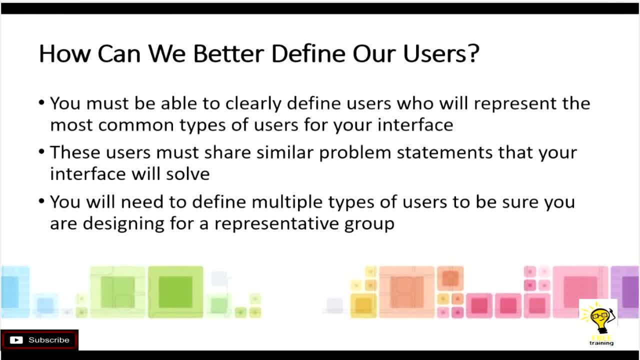 doesn't think of it the same way you do, or no matter what you did, it's not quite right. And that's where the iterative design process comes in. that allows you to modify your design and go back to the user with a new approach so you can see if that works for that specific user. 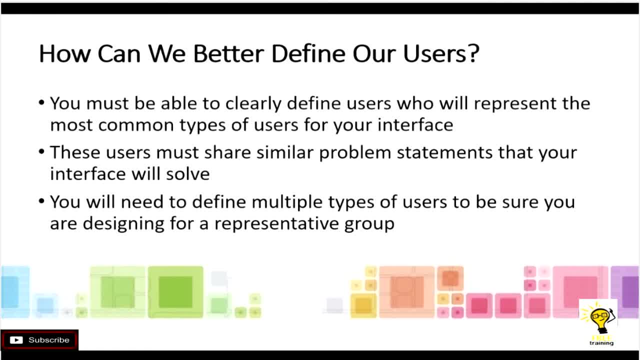 But that is a little bit of information about defining the user and things to keep in mind when doing so. Later in the course, we'll take a look at some of the tools you can use to assist you in coming up with those specific users that you're going to design for. So that is information. 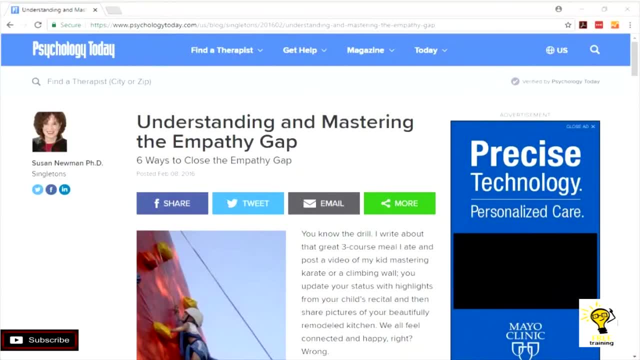 about defining the user. In this lesson, I want to familiarize you with a term in psychology called the empathy gap, And what I'm going to show you is an article by Susan Newman in Psychology Today magazine, talking about the empathy gap. Now, the focus of this article is just a little bit different. 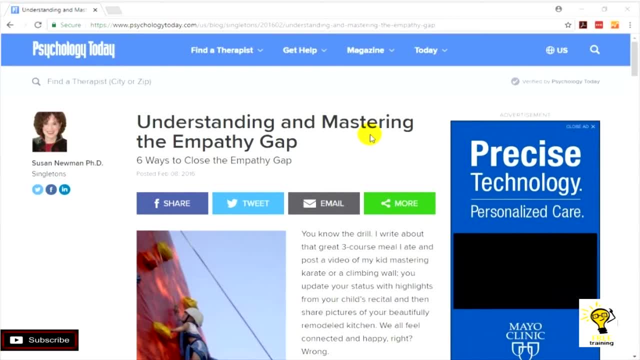 than the focus I'm going to take with it, But the idea is we are a designer trying to design for a user And we're going to talk about how to design for a user And we're going to talk about how to design for a user And we're going to talk about how to design for a user And we're supposed 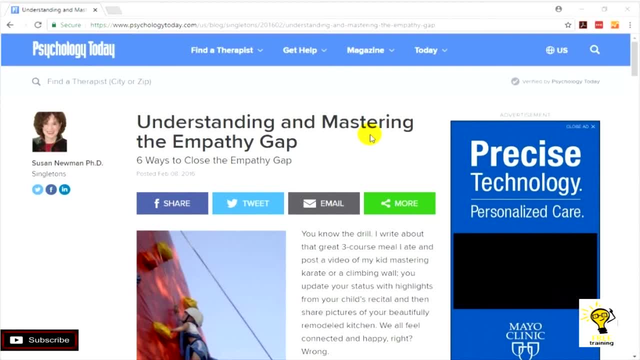 to keep the user at the center of that process, But we've already spoken about the fact that we cannot truly be the user and understand them. So we have to accept the fact that our understanding of them will not be perfect, And the space between their actual experiences and ours is known as the 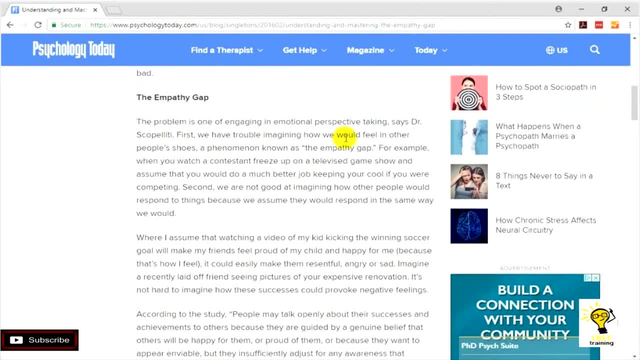 empathy gap And there's a good example in this article talking about it, And this phenomenon is known as the empathy gap And they have a great example in here: When you watch a contestant freeze up in a televised game show and assume you would do a. 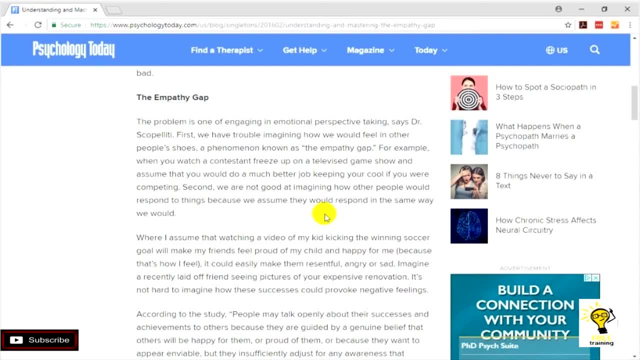 much better job keeping your cool if you were the one competing. that difference is known as the empathy gap. You can't truly empathize by the user because you are not them and you're not there at that exact moment in time experiencing what they are. We are also. 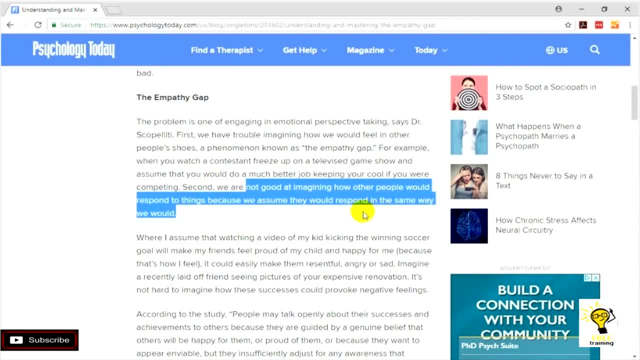 not good at imagining how other people would respond to things, because we assume they'd respond in the same way we would. That comes into play when you are creating your design, because you always assume, as a designer- and there's nothing wrong with this- that your design 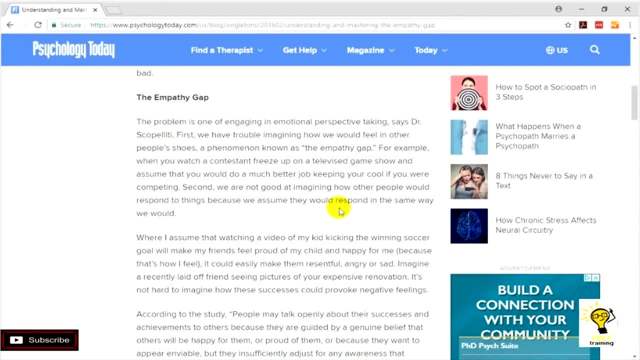 is the best design you can do, so other people should like it, appreciate it and be able to work with it. So it's something to keep in mind. I just wanted to bring up this concept because there is a gap between individuals, no matter how close they think they are to understanding the other. 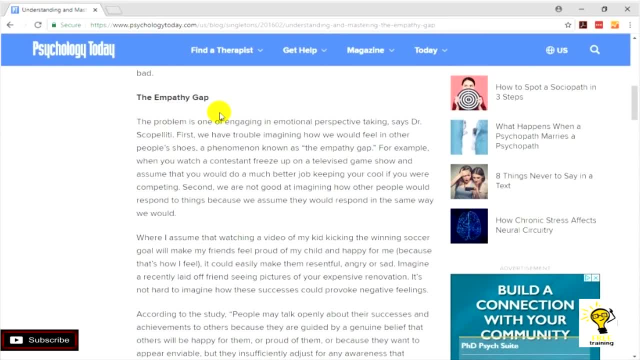 person. There's always this little bit of empathy gap between them and sometimes that empathy gap is a little more than just empathy, It's much larger. So if you create and design something for a user and the user goes in to use it and is unhappy with it, that's because that empathy gap is a little bit too wide between you. 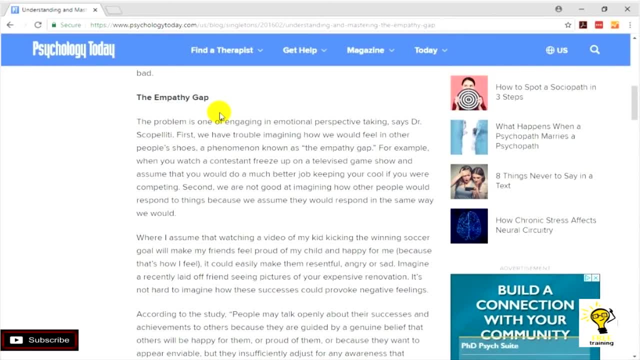 and the user, So just keep that in mind. The point of this lesson was just to familiarize you with this concept, and it is an official concept within psychology, So it's one we have to specifically agree with, because it's done based on research, And keep it in mind, especially if 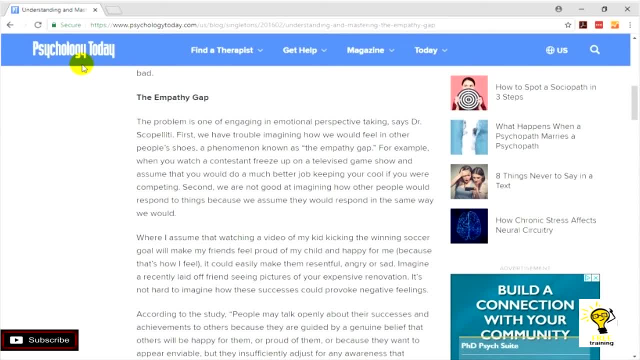 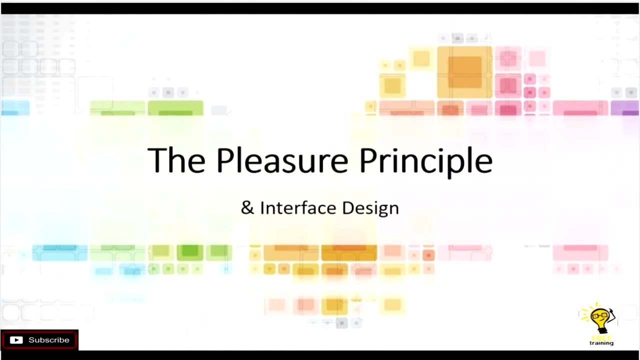 your users are not responding the way you thought they would when you go to work with them and test your designs. So that is the empathy gap in psychology. In this lesson we're going to talk about the pleasure principle and interface design, And it sounds like a rather odd combination. 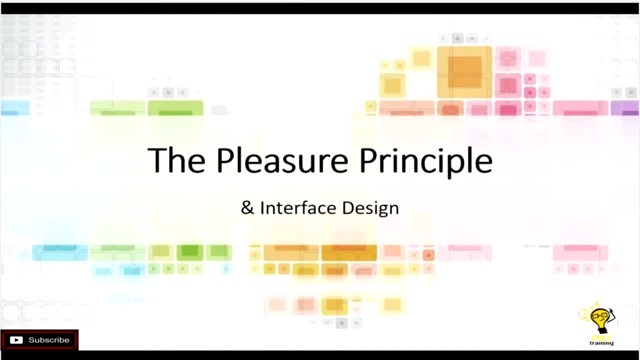 but it's not. So let's get started. But there's a lot of human psychology in how users behave and interact with interface design. So some of these different principles are very valuable in assisting you in designing for the user. So let's take a look at the pleasure principle. This is a term originally used by 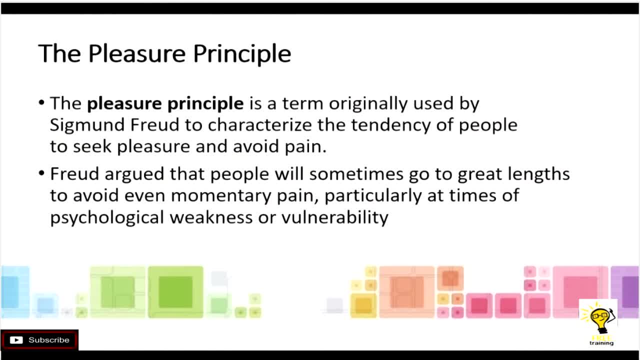 Sigmund Freud. Most people have heard of him, even if they're not in the psychology field. He used this to characterize the tendency of people to seek pleasure and avoid pain. He argued that people will sometimes go to great lengths to avoid even momentary pain. 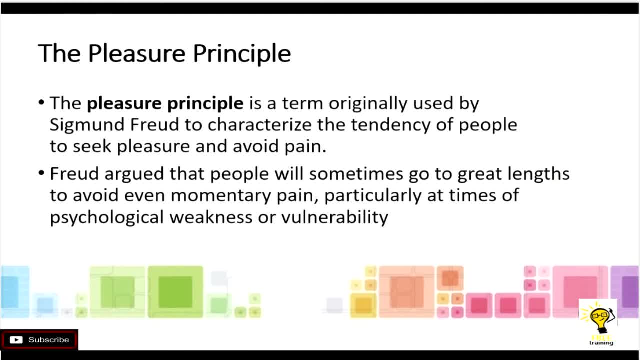 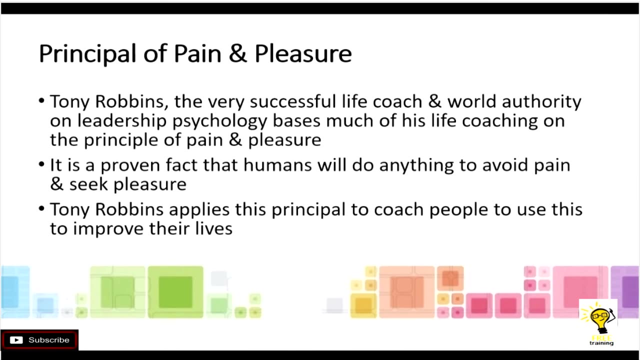 particularly at times of psychological weakness or vulnerability. Now, Freud is known for going to the extreme of his specific concepts, But the basics of this principle still apply to human nature. Tony Robbins, the very successful life coach and world authority on leadership psychology. 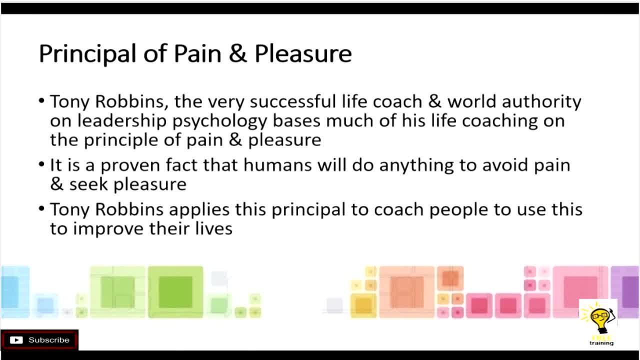 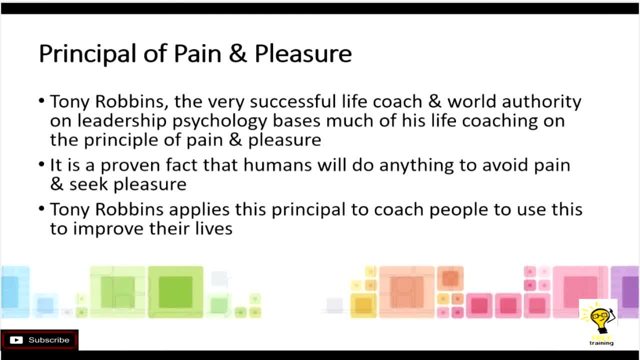 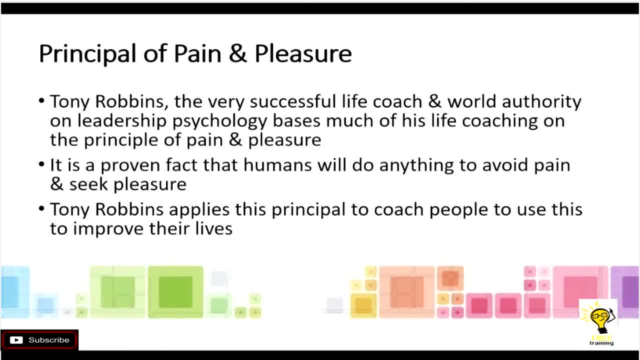 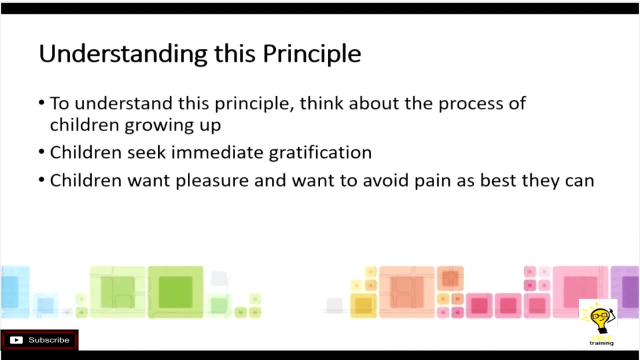 and what's pleasurable, But Tony Robbins applies this principle to coach people to use this to improve their lives. Sometimes it's just their perception of pain versus pleasure that is the problem. So how can this help us in interface design If you think about the process of children growing up? 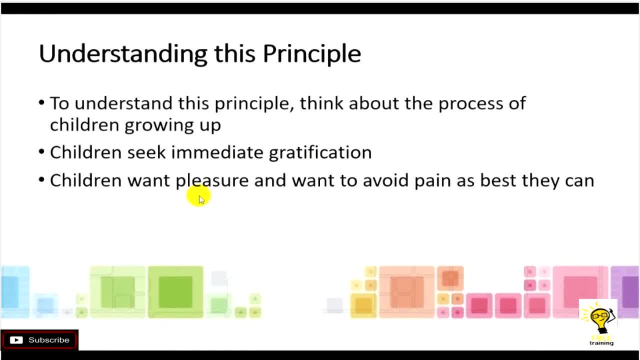 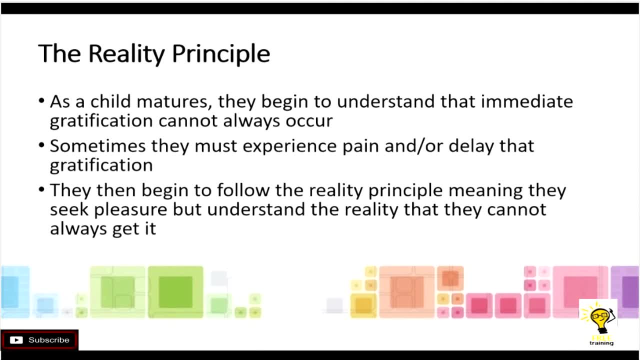 they seek immediate gratification. Children want pleasure immediately and want to avoid pain as best they can. As we mature, or as a child matures, they begin to understand that immediate gratification cannot always occur, And that is when the reality principle comes into play. Sometimes they must experience pain and or delay. 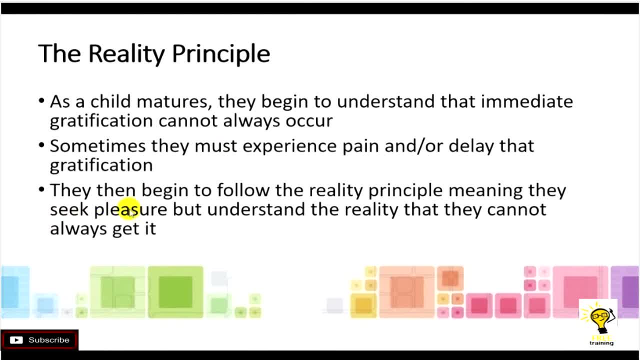 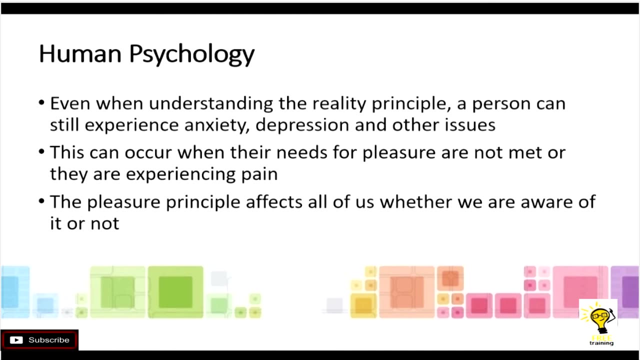 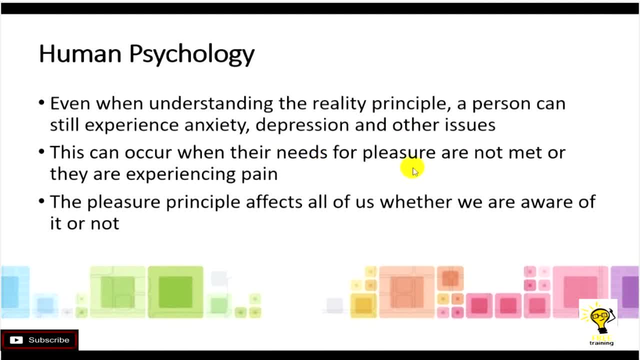 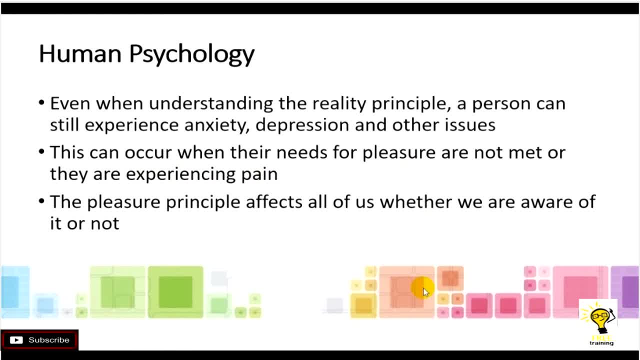 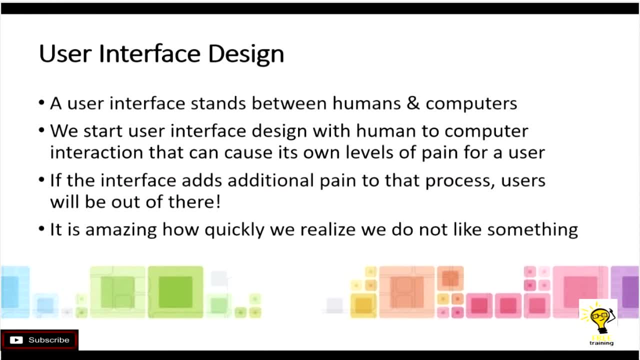 going to trigger their experiencing of pain and they will not like the interface. A user interface stands between humans and computers. We start user interface design with human to computer interaction and that alone can cause its own levels of pain for a user. So if the interface adds additional pain, 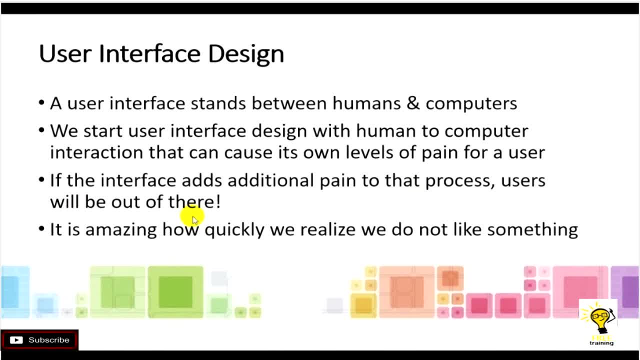 to that process. users will be out of there, And I think we can all relate to that fact. It's amazing how quickly we realize we do not like something, So keep that in mind as you are creating your user interface design. Humans will avoid pain and move towards pleasure. 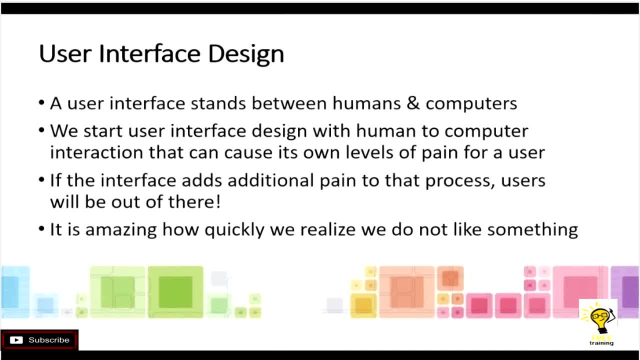 You want to make sure that the tasks can be accomplished in a pleasurable way for the user, And we're going to take a look at that in another lesson. Just keep in mind that the pain pleasure principle- avoiding pain, seeking pleasure- has an effect on everything. 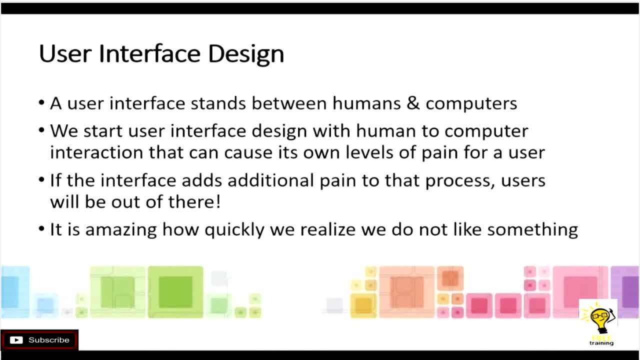 we do in human behavior And factor that in to your user interface design concepts. Make sure that you are focusing on the pleasurable side of things and making sure that the user avoids pain when they're using your interface. So that's some information about the pleasure principle. 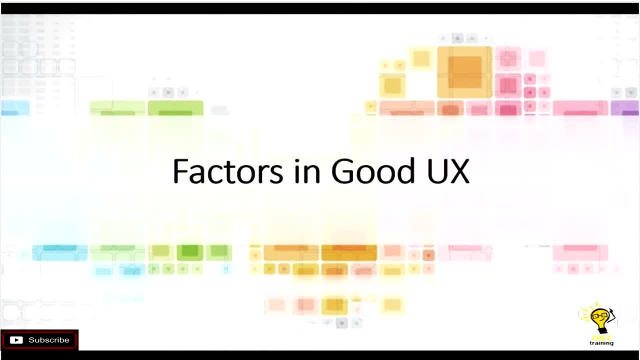 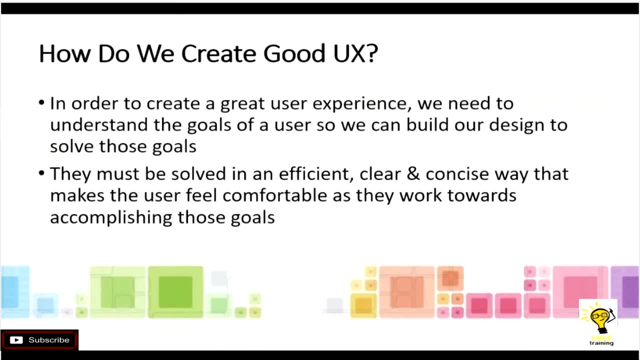 So what are the factors in good UX? That's what we're going to take a look at in this lesson. So how do we create good UX? In order to create a great user experience, we need to understand the goals of a user. 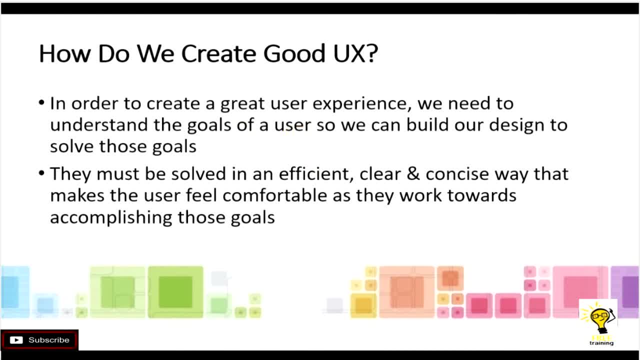 And that is the main focus of any type of UX. That way, we can build our design to solve those goals. Now they must be solved in an efficient, clear and concise way that makes the user feel comfortable as they work towards accomplishing those goals. 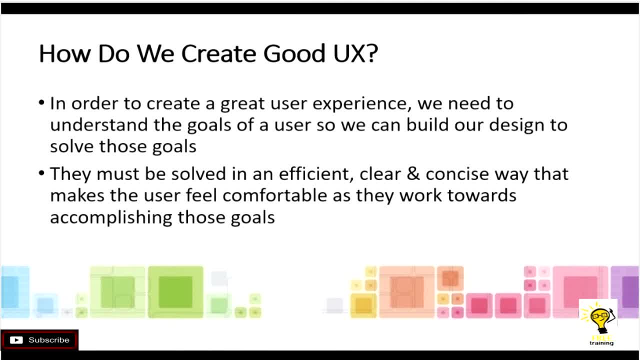 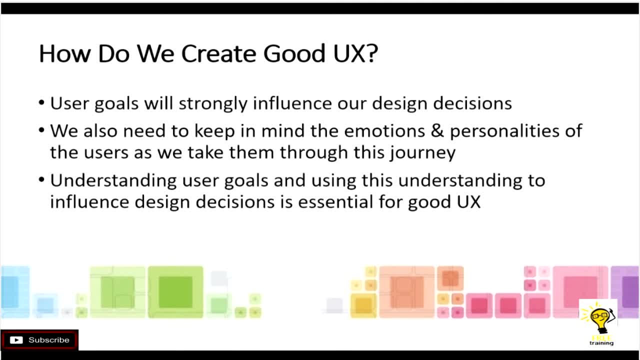 And if you think about any type of user interface, frustrations occur when they cannot accomplish those goals. User goals will strongly influence our design decisions. We need to make sure that they are able to accomplish these goals. We also need to keep in mind the emotions and personalities. 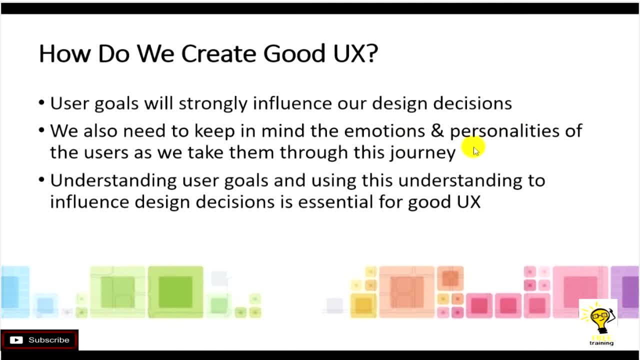 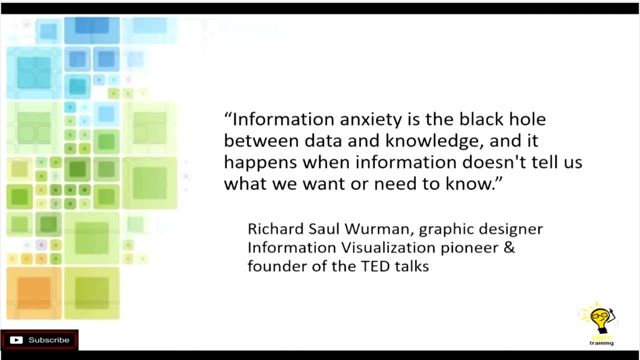 of the users as we take them through this journey. Understanding user goals and using this understanding to influence design decisions is a essential for good UX. It just makes sense. Here is a great quote from Richard Saul Wurman. He's a graphic designer- information visualization. 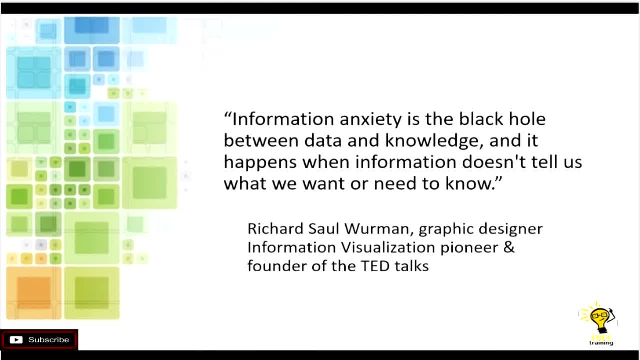 pioneer and he founded TED Talks. Information anxiety is the black hole between data and knowledge, And it happens when information doesn't tell us what we want or need to know. Now, if you apply that to the user interface, notice the word anxiety. 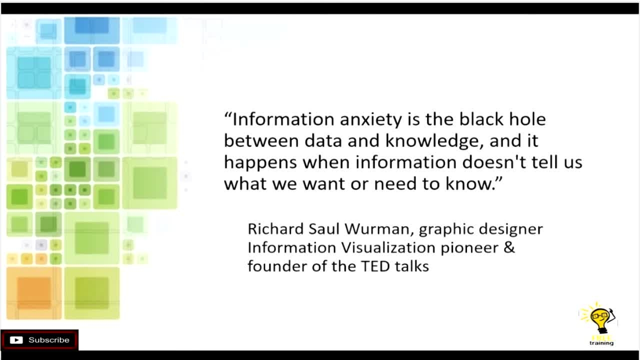 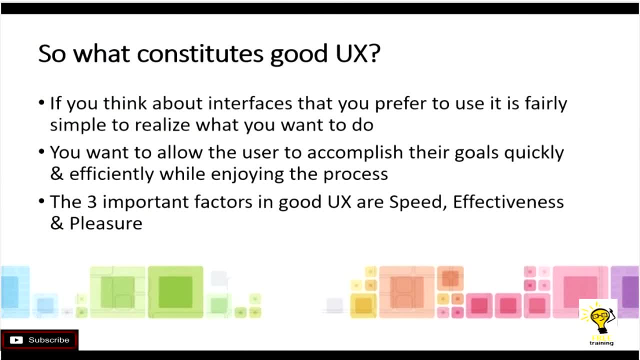 That starts to creep up if the user has difficulty accomplishing their goals. So what constitutes good UX? If you think about interfaces that you prefer to use, it's fairly simple to realize what you want to do. What you want to do is allow the user to feel comfortable, aiming to be good. 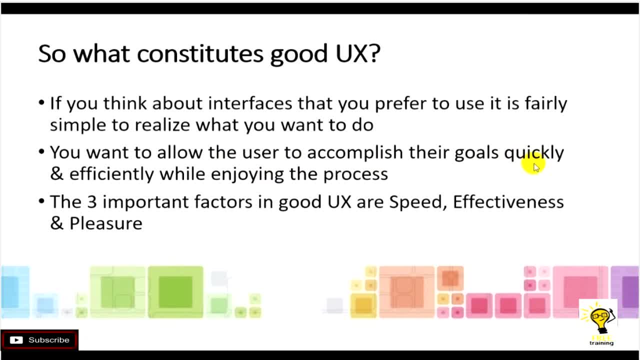 What you want to do is allow the user to feel comfortable, aiming to be good, the user to accomplish their goals quickly and efficiently while enjoying the process. Oh, it sounds so simple. The three important factors in Good UX are speed, effectiveness and pleasure. 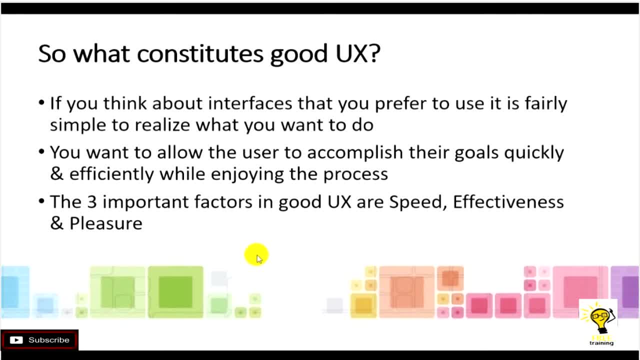 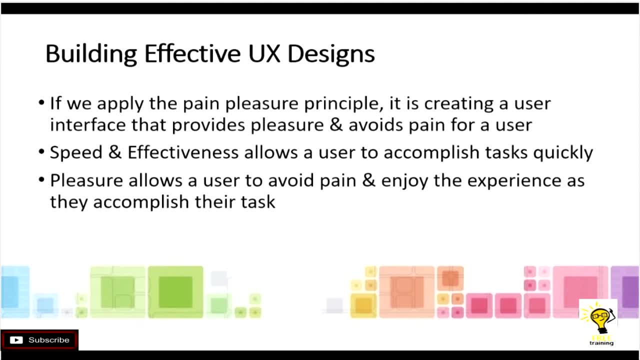 And included in that pleasure is avoiding pain. If we apply the pain pleasure principle, it's creating a user interface that provides pleasure and avoids pain for the user. Speed and effectiveness allows a user to accomplish their tasks quickly. Pleasure allows a user to avoid pain and enjoy the experience. 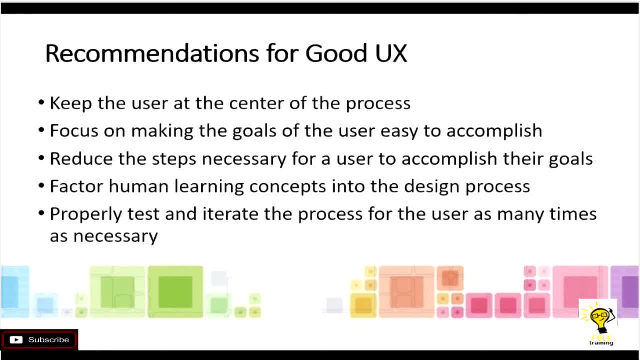 as they accomplish their task. So what are some recommendations for Good UX based on all of that information? Keep the user at the center of the process. The user is the center. Focus on making the goals of the user easy to accomplish And in order to do that, we want to reduce. 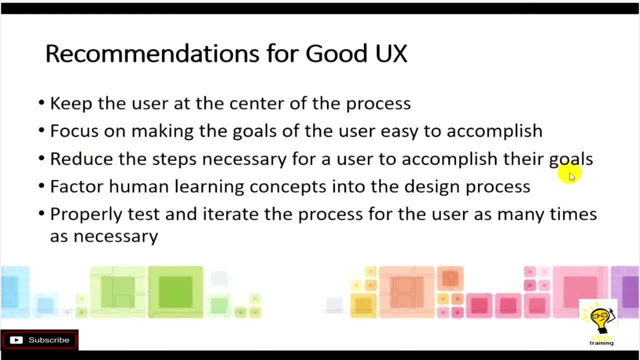 the steps necessary for a user to accomplish those goals. Factor human learning concepts into the design process, And that's what I've tried to incorporate for you within this course: Properly test and iterate the process for the user as many times as necessary, even if it's well. 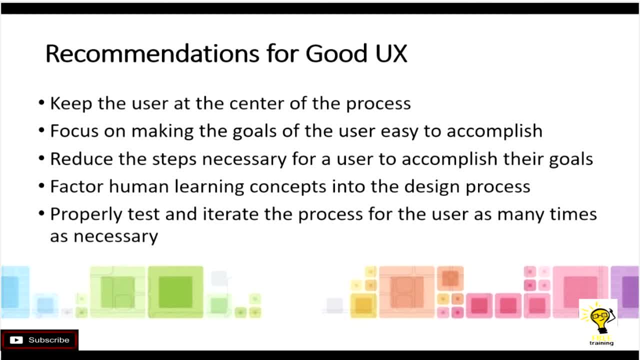 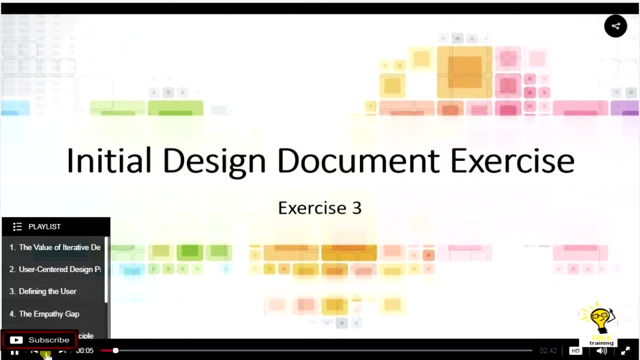 beyond what you originally thought you would need to do. So those are factors in Good UX and some specific recommendations for accomplishing that. For those of you taking this course as a workshop course, it's time for exercise three. In this exercise, you're going to create what I call an initial design. 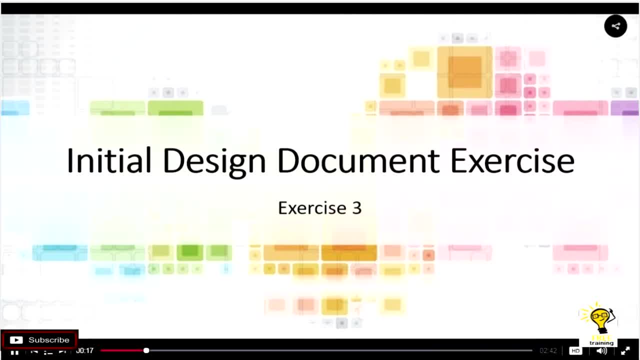 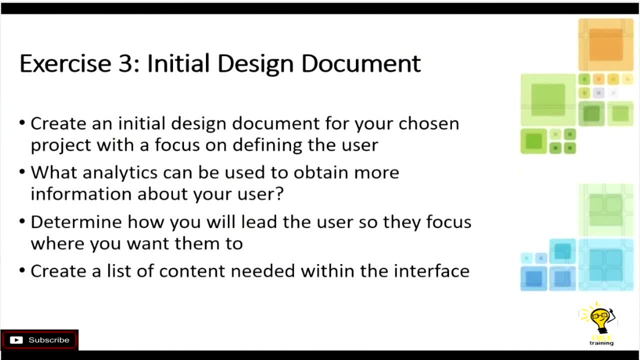 document. So let's take a look at what that should contain. You're going to create an initial design document for your chosen project that you created in an earlier exercise with a focus on defining the user. So, in order to define and document that user definition, 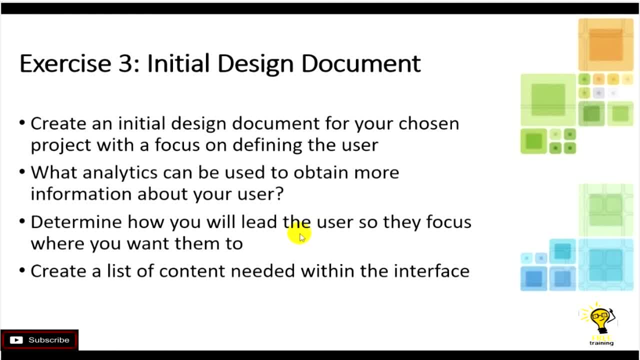 you can answer or explore the following questions: What answers do you want to answer? What do you seek to implement? What may you recommend that they do? What are the actions you're acting to take so they're following in your practice? A tip that needs working with the client. 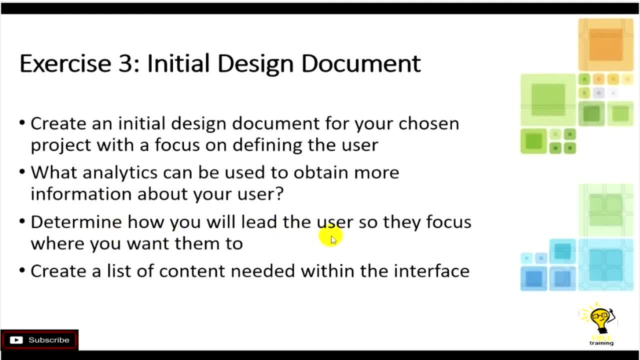 is to know about understanding the definition and the spirit of the idea that you're providing. If you're provided with the service of doing things for your user, do you know and understand in a way that you can use the service as a goal to determine how they will小? 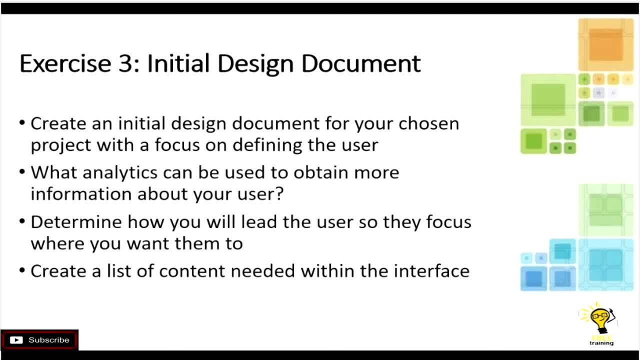 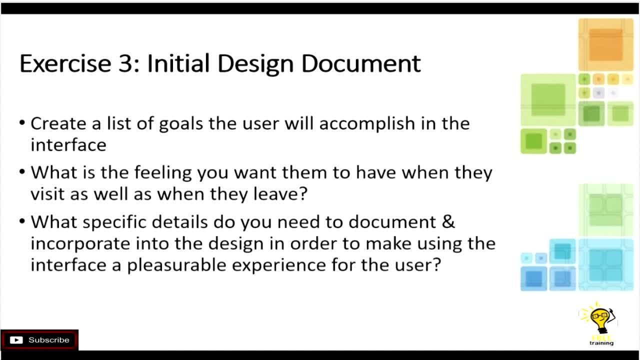 an outcome. in a project, The communication is critical. for instance, Consider and take into account when you do go to actually create the design. Create a list of goals the user will accomplish in the interface. What is the feeling you want them to have when they visit?